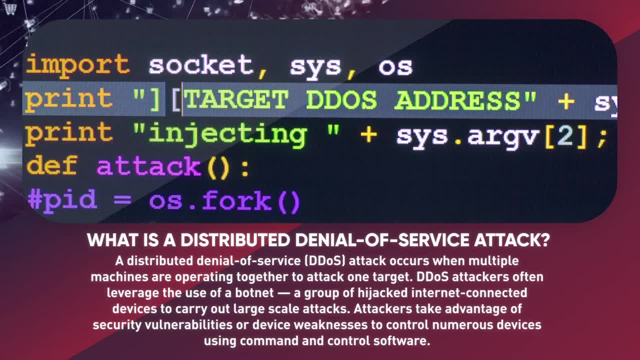 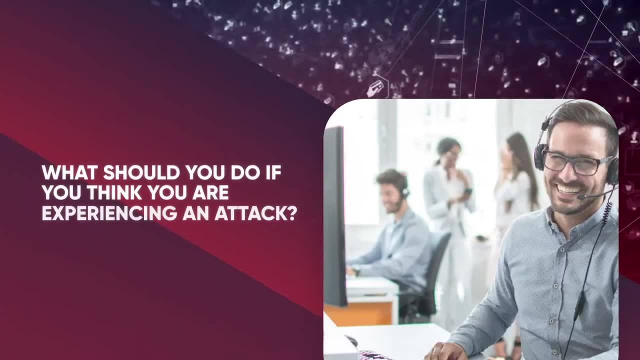 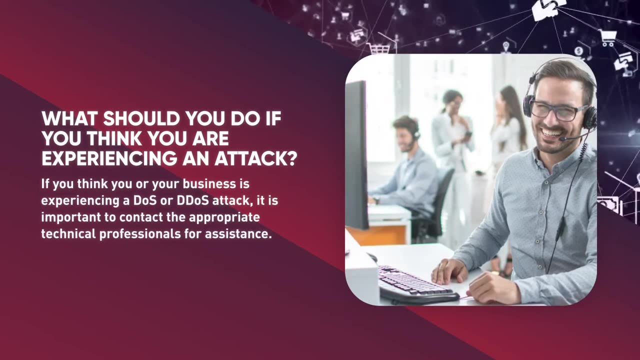 Attackers take advantage of security vulnerabilities or device weaknesses to control numerous devices using command and control software. If you think you or your business is experiencing a DOS or DDoS attack, it is important to contact the appropriate technical professionals for assistance. Tutorial 13: Routing Services. 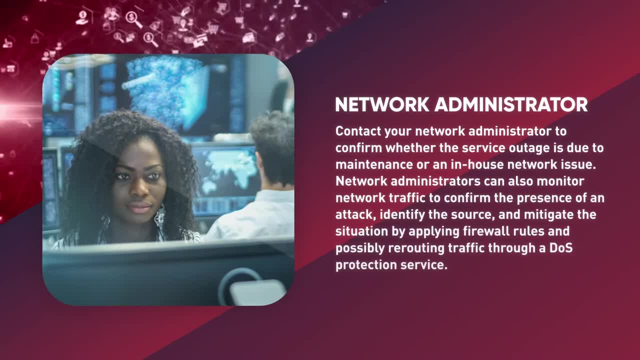 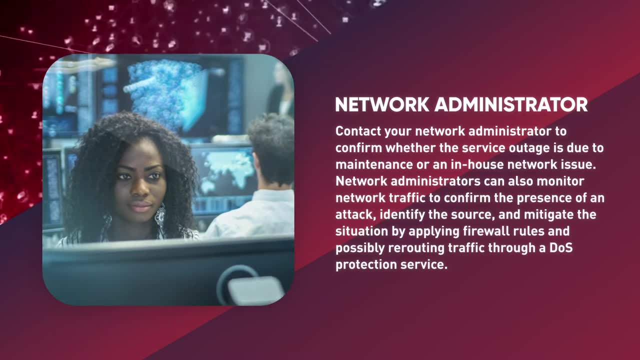 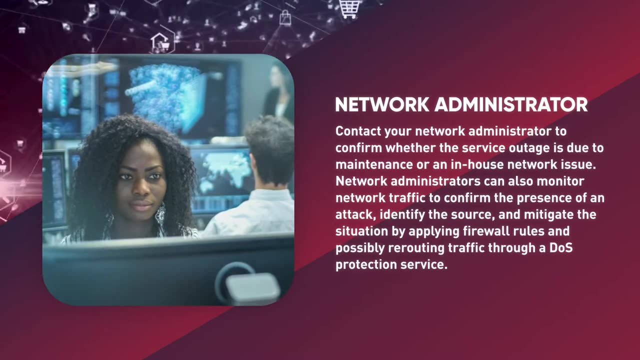 Contact your network administrator to confirm whether the service outage is due to maintenance or in-house network issues. Network administrators can also monitor network traffic to confirm the presence of an attack, identify the source and mitigate the situation by applying firewall rules and possibly rerouting traffic through a DOS protection service. 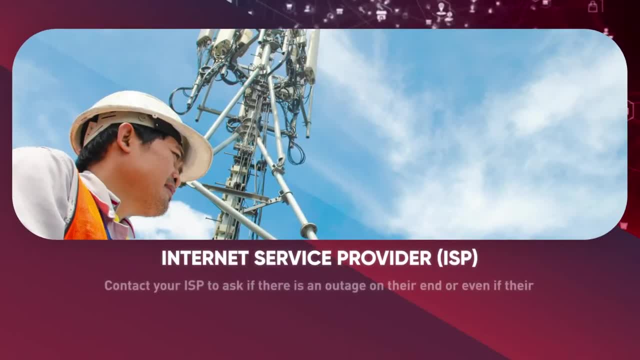 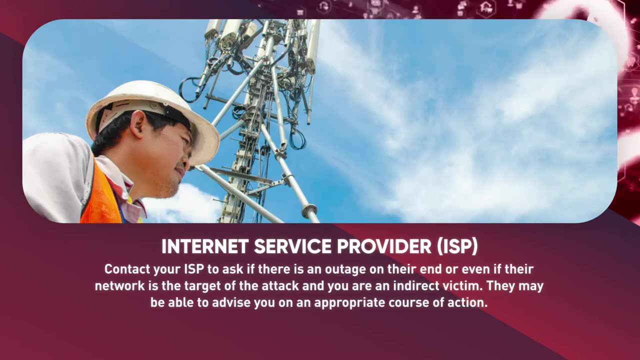 Tutorial 24: Bestyle your network. Contact your internet service provider or ISP to ask if there is an outage on their end or if there is a troubleshooting. Tutorial 25: goverment services and other services havemagic capabilities. even if their network is the target of the attack and you are an indirect victim, they may be able to. 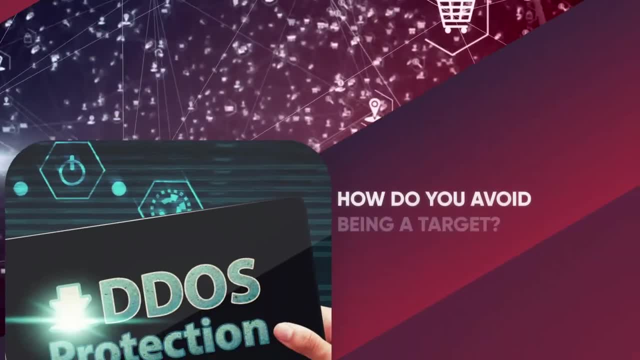 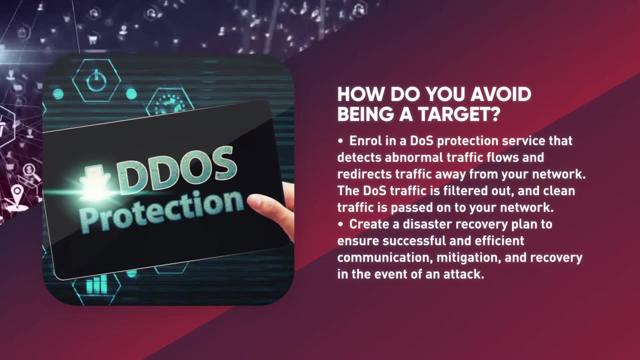 advise you on an appropriate course of action. how do you avoid being a target? while there is no way to completely avoid becoming a target of a dos or ddos attack, there are protective steps administrators can take to reduce the effects of an attack on their network. enroll in a dos. 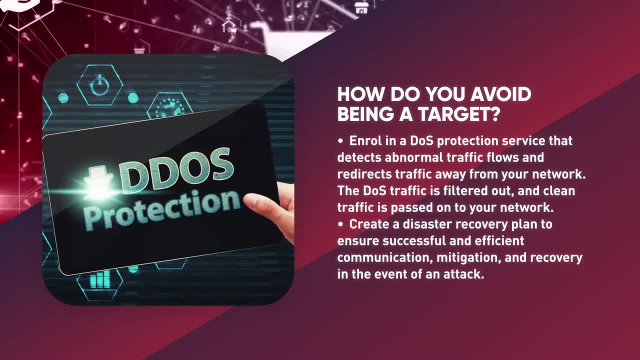 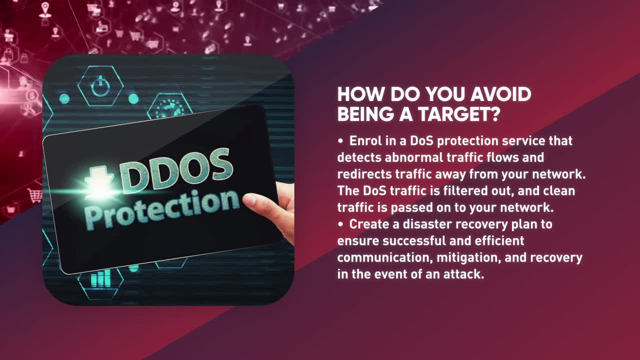 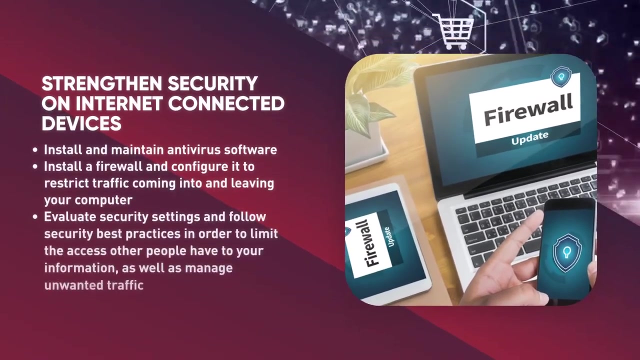 protection service that detects abnormal traffic flows and redirects traffic away from your network. the dos. traffic is filtered out and then clean traffic is passed on to your network. create a disaster recovery plan to ensure successful and efficient communication, mitigation and recovery in the event of an attack. strengthen security on internet connected devices. it's also important. 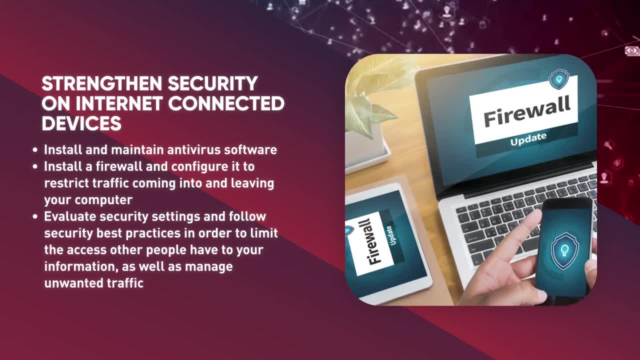 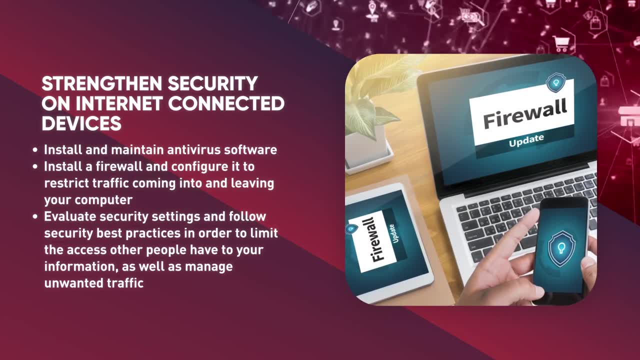 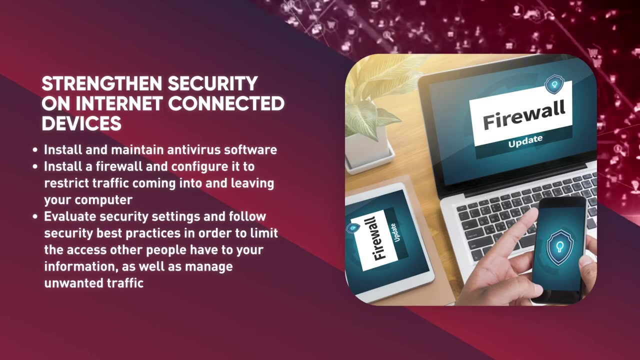 to take steps to strengthen the security posture of all of your internet connected devices in order to prevent them from being compromised. install and maintain antivirus software. install a firewall and configure it to restrict traffic coming into and leaving your computer. evaluate security settings and follow security best practices in order to limit the access. 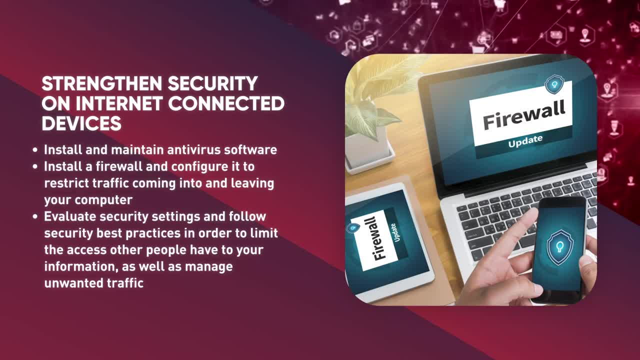 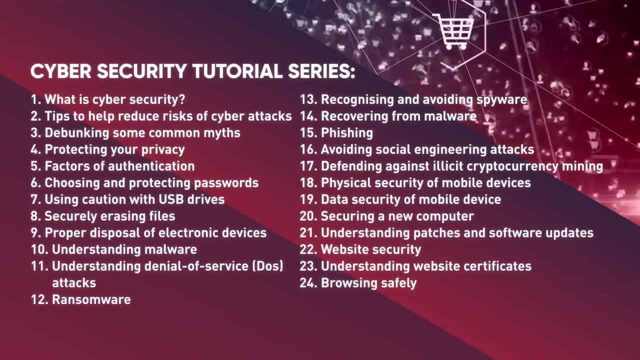 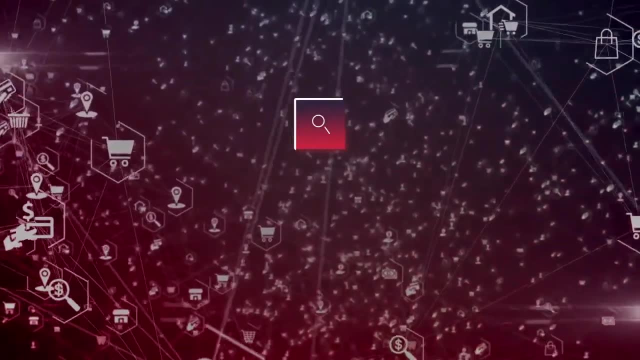 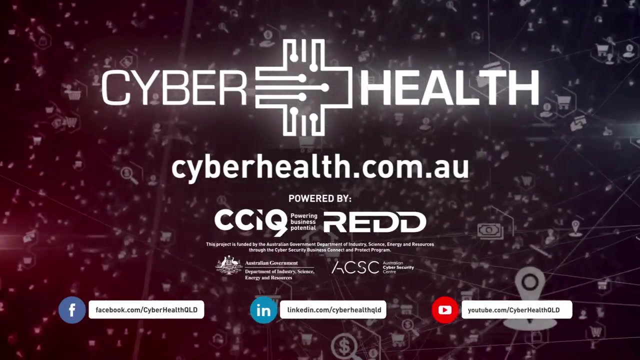 other people have to your information, as well as manage unwanted traffic. check out more videos from this cyber security tutorial series to learn how you can better protect your information and devices from cyber attacks. cyber health is powered by the chamber of commerce and industry queensland and red.